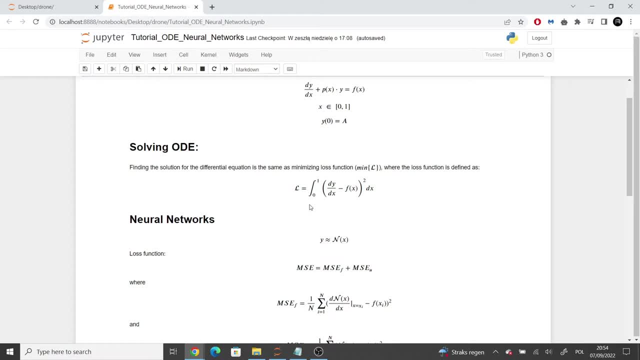 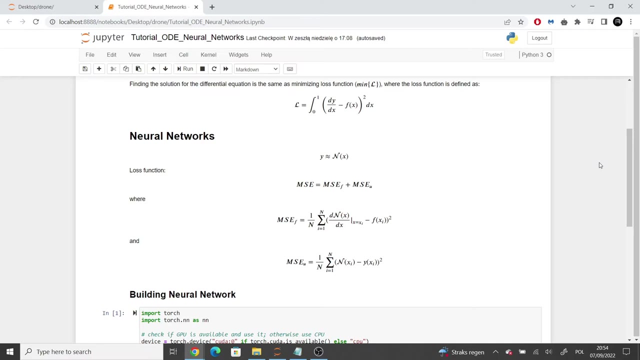 Because minimizing the loss function is equivalent to solving the differential equation, it is possible to teach the neural nets to predict the solution of the equation. The output of the solution is the same as the solution of the equation. The output of the neural network will represent the solution y. The integral loss function will be defined. 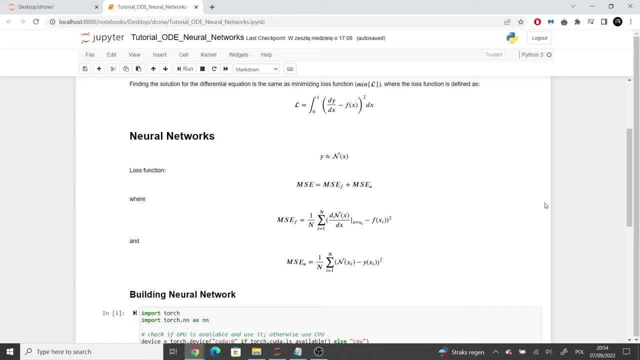 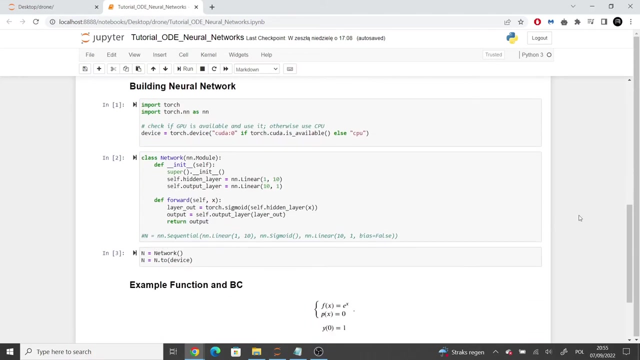 using the mean squared error. The loss function is split into two parts. One is based on the differential equation and is referred to as MSEF, And the second one is based on the boundary conditions and is referred to as MSEU. So first we must define the neural network. This network will have one hidden layer and 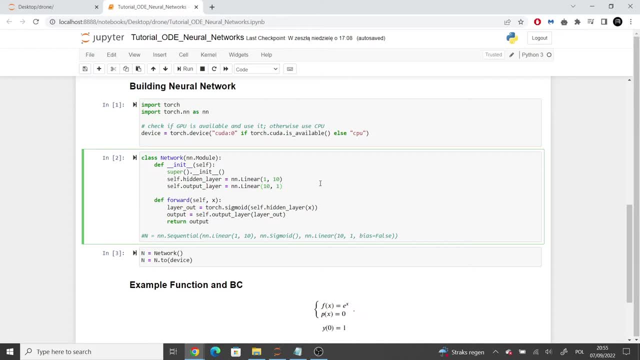 the sigmoid function is used for the activation. Of course this can be programmed using one line of code shown here in the comments, Of course without the bias. But of course it is good to practice The more formal way of coding the neural networks in PyTorch. 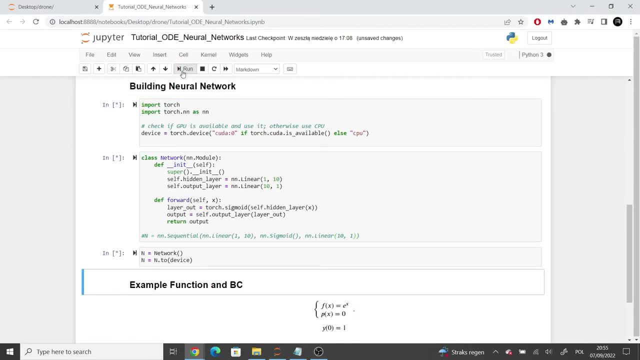 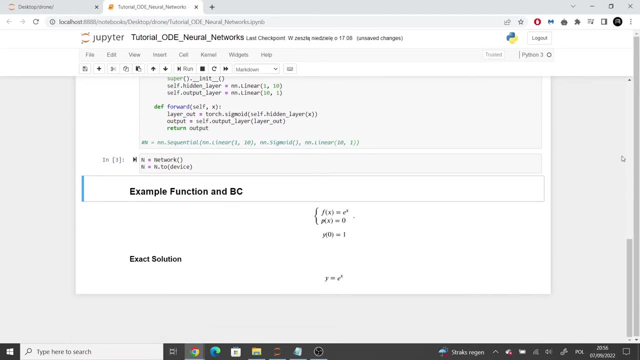 So let's run these lines. The first example of ODE is defined as the following: So the ODE is simply: y prime equals to e to the power of x, And because the boundary condition at the x equals 0 is 1.. The exact solution to this equation is: y equals e to the power of x. 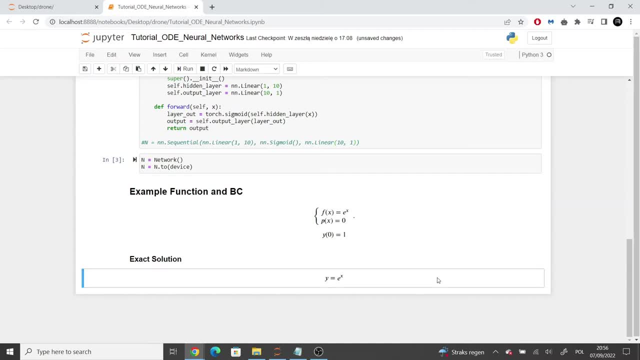 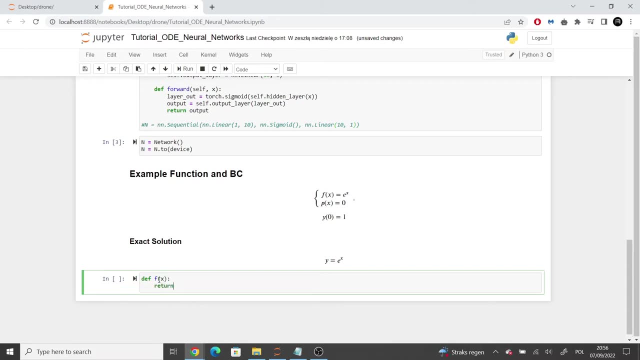 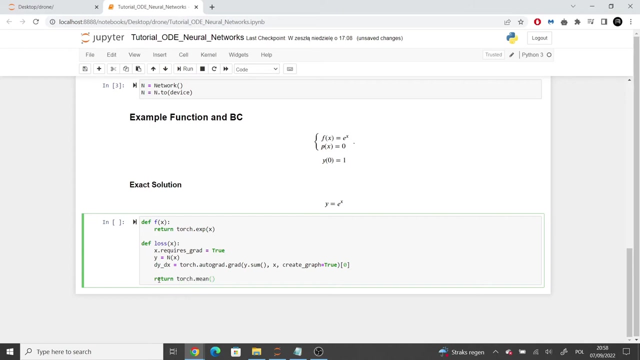 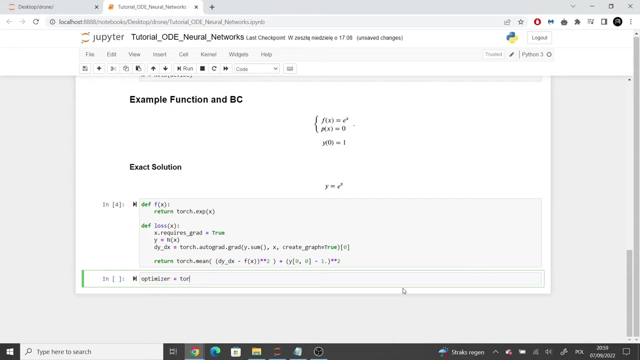 First let's define the function f and the loss function. Let's verify the function f and the loss function. Now we can run this cell and define the optimizer and train the neural network using the back propagation. For the optimizer I decided to use the LBFGS optimizer. 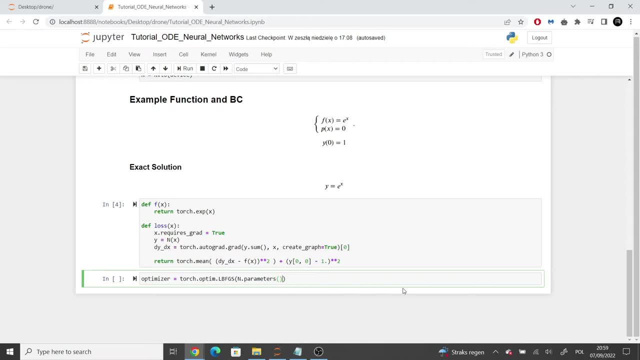 I will not explain how this optimizer works. If you are interested, then you can read about it on your own. I will also share a link to the article in the description. If you want, you could also use a different optimizer, such as the Adam optimizer, which. 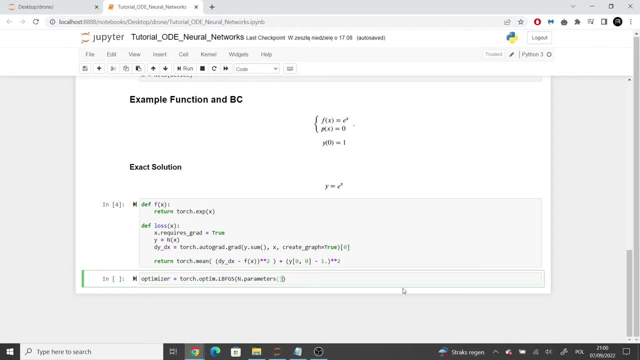 of course, is a bit simpler, But then you should keep in mind that it requires more epochs, about 10,000.. In this case, we can simply use the LBFGS optimizer. I will use 10.. So let's train the model. 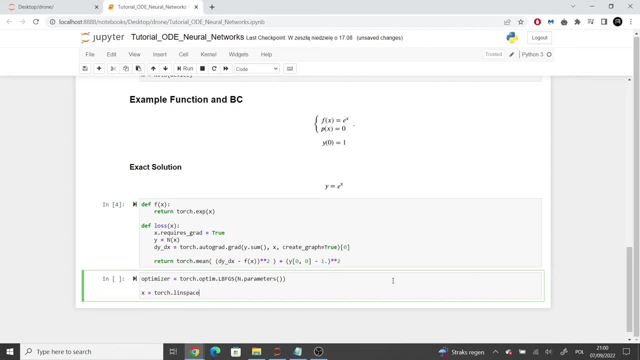 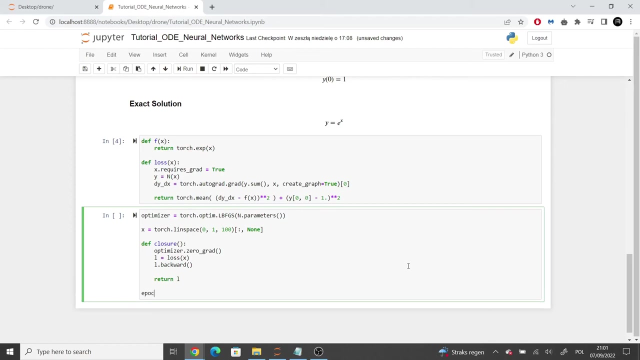 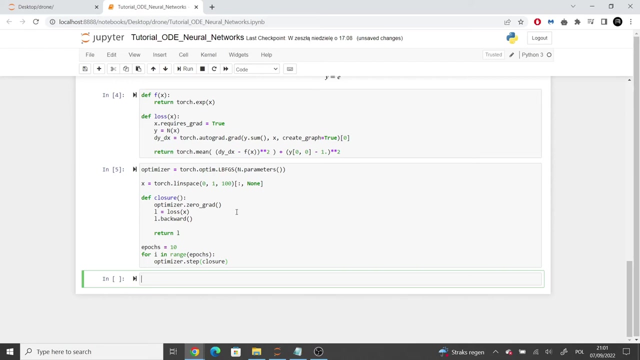 Okay, so let's train the model. Okay, so, let's train the model. Okay, so, let's train the model. Lastly, we can predict the full solution using the trained Neuralet and compare the solution, the predicted solution, to the exact solution. 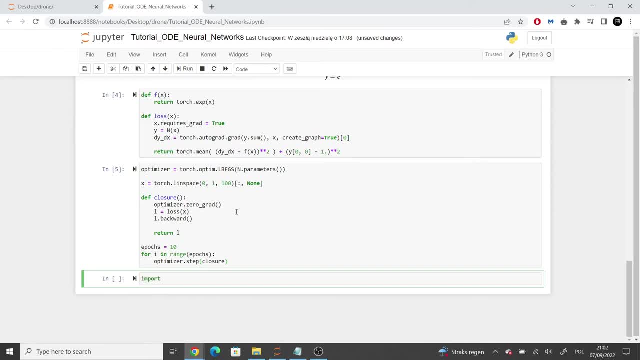 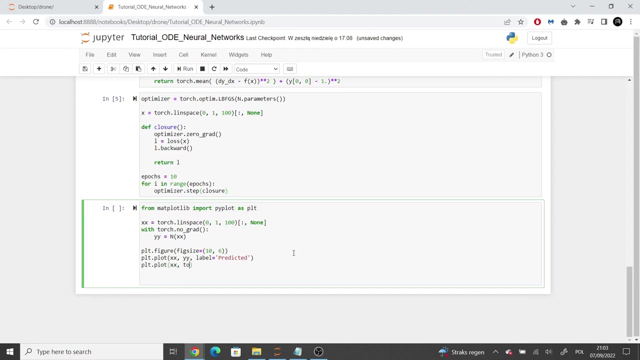 So let's import the pi plot from matplotlib. Now we can compute y using matplotlib. Next, we can compute the value of the neural network and plot the results. Next, we can compute the value of the neural network and plot the results. Thank you.